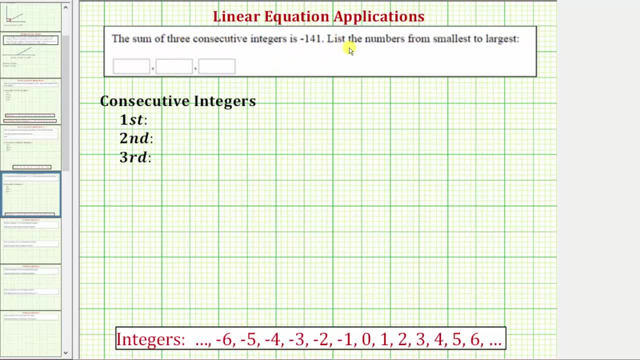 The sum of three consecutive integers is negative 141.. We're asked to list the numbers from smallest to largest. A list of consecutive integers is given here below. Notice how, as we list the integers from left to right, they increase by one each time. 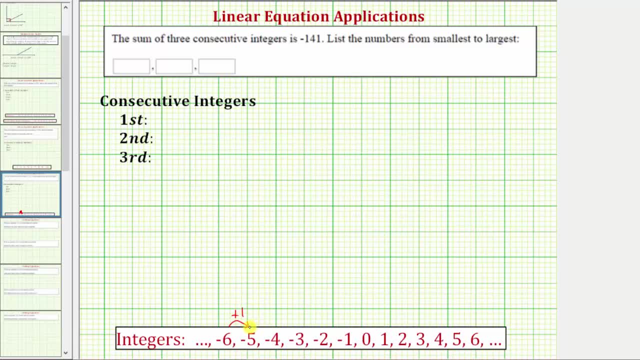 Negative six plus one equals negative five. Negative five plus one is negative four. Negative four plus one is negative three, and so on. Because of this, if we let the first consecutive integer be equal to x, the next consecutive integer would be x plus one, followed by x plus one plus one. 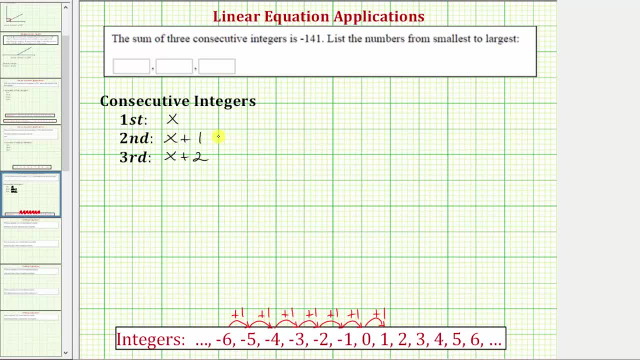 or x plus two. And now, because we know the sum of these consecutive integers equals negative 141,, we can measure an equation, solve for x and determine the consecutive integers. The equation would be: x plus x plus one plus x plus two equals negative 141. 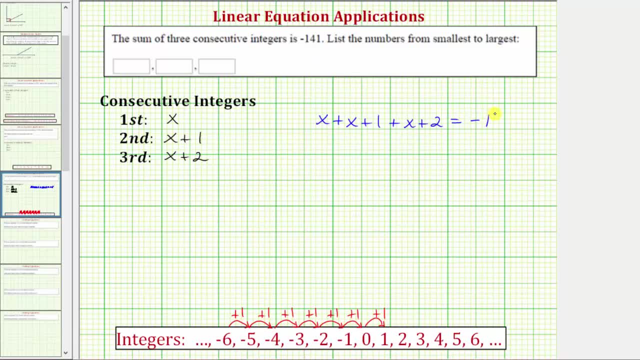 The equation would be: x plus x plus one plus x plus two equals negative 141.. Let's simplify the left side of the equation: X plus x plus x equals three. x And one plus two equals three. So the left side simplifies to three: x plus three. 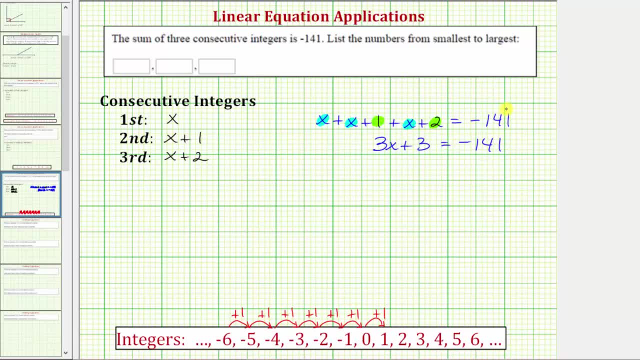 and this equals negative 141.. Now we have a basic two-step equation to solve. Now we have a basic two-step equation to solve. Now we have a basic two-step equation to solve. The first step is to add or subtract, to isolate the variable term. 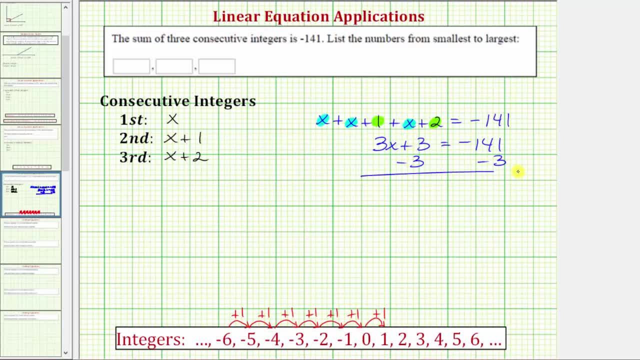 To undo plus three, we subtract three on both sides. Simplifying subtracting three undoes plus three or three minus three is zero. So we have three x equals negative 141, minus three equals negative 144.. And now we multiply or divide to solve for x. 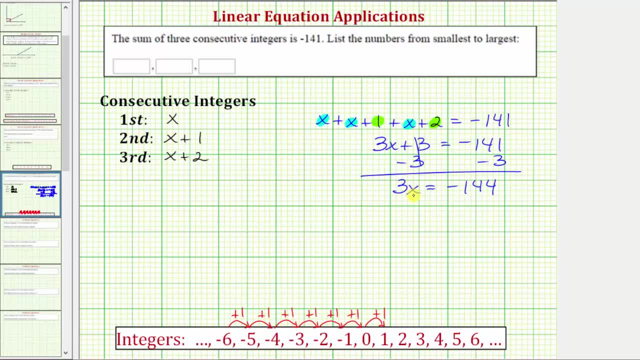 And because three x means three times x, to undo this multiplication we divide both sides by three. Dividing by three undoes multiplying by three. So the left side simplifies to x, Or three divided by three is one. One times x is x.